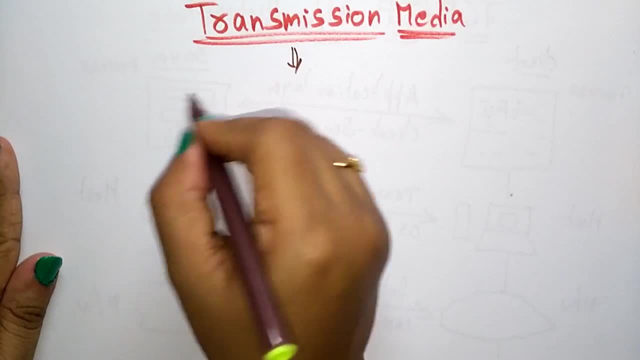 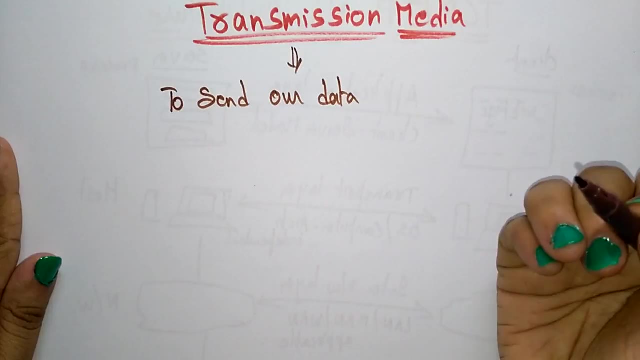 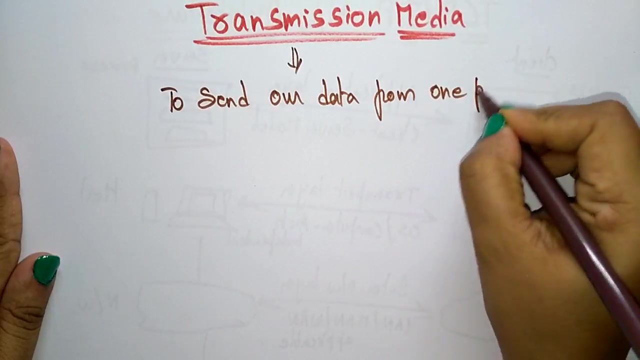 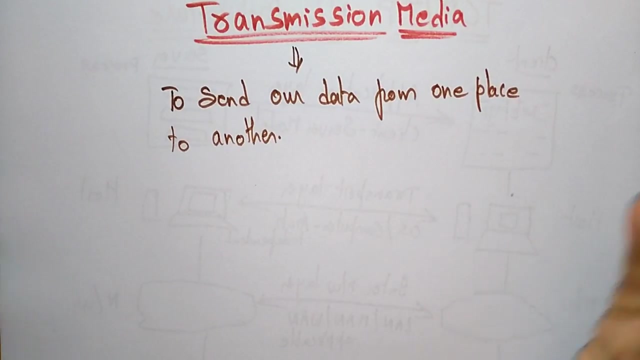 It is a means to send our data. A data may be any type, It is a voice or message, whatever it may be- To send our data from one place to another place, From one place to another. So the first layer, that is a physical layer. 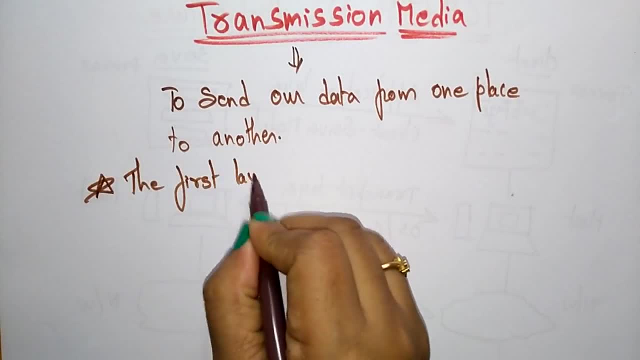 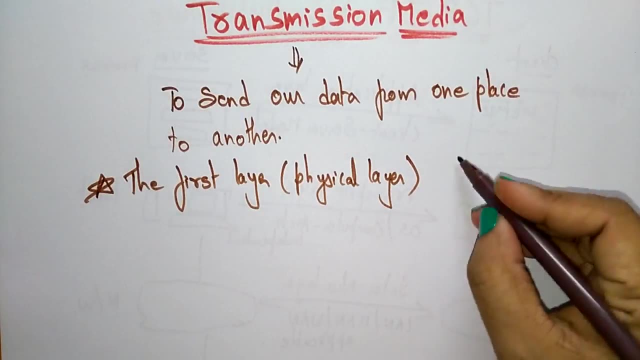 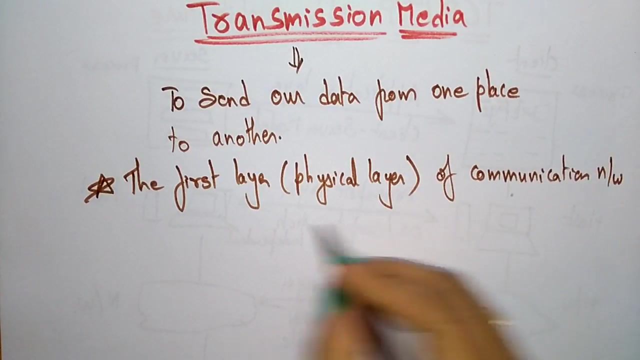 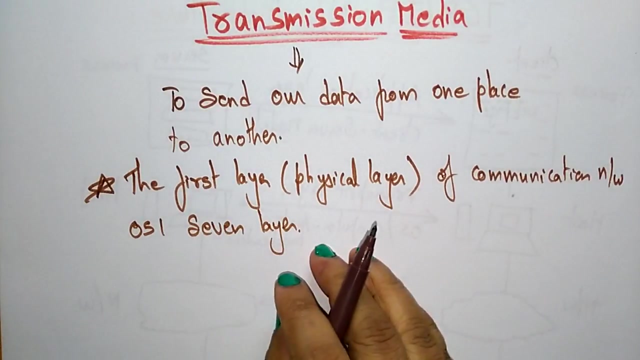 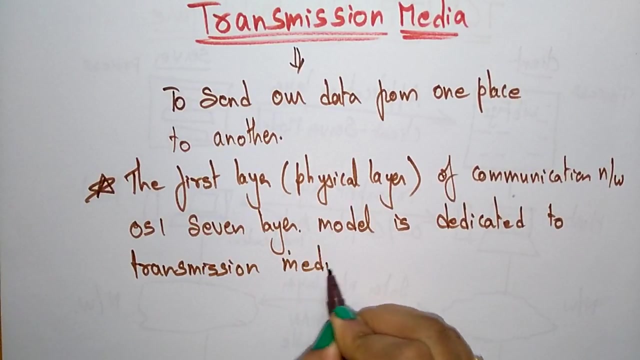 The first layer, That is a physical layer of communication, of communication network, OSI seven layer. So if you take in the OSI seven layer, the first layer that is present is the physical layer. So this physical layer model is dedicated to transmission media, transmission media. 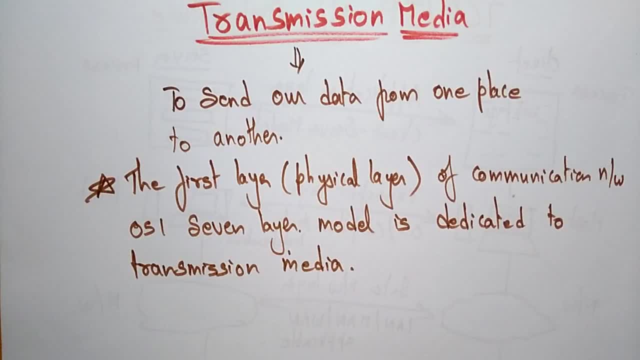 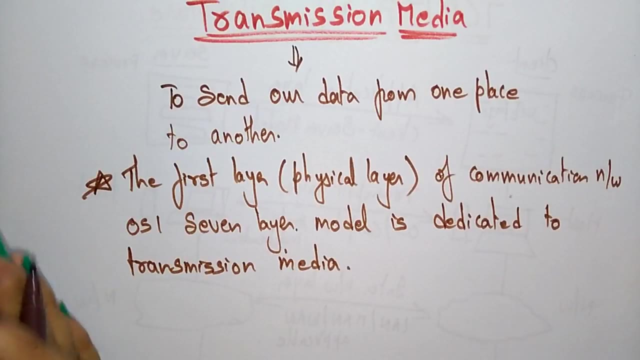 So the most, the first layer that is present in the layer whatever, the OSI seven layer, or you can take the TCP IP layer. So this seven layer, this physical layer, is mainly dedicated to the transmission media, So that is only. it is sending the data from sender to the receiver. The sender is sending the data to receiver with the help of physical layer. the last, first layer. 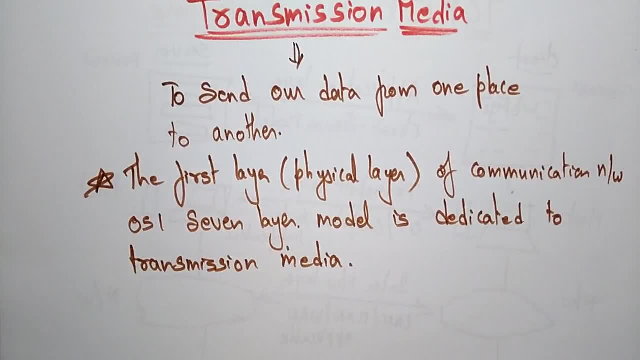 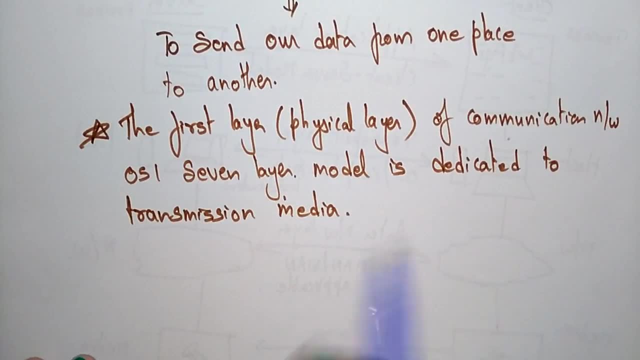 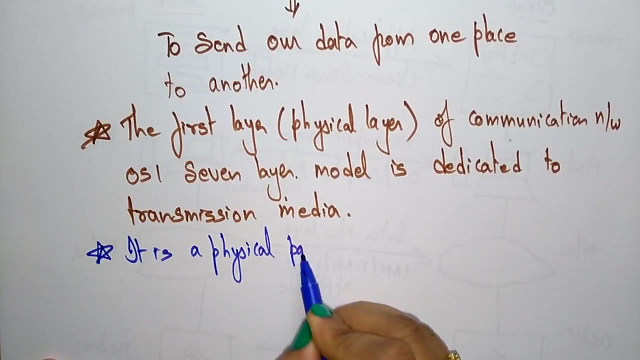 And from the receiver side, the physical layer is accepting the data from sender. So it is a physical path. You just call it as it is: a physical path between. It is a physical path, Maybe a physical, or sometimes it acts as a physical, or sometimes it acts as a just a wireless. 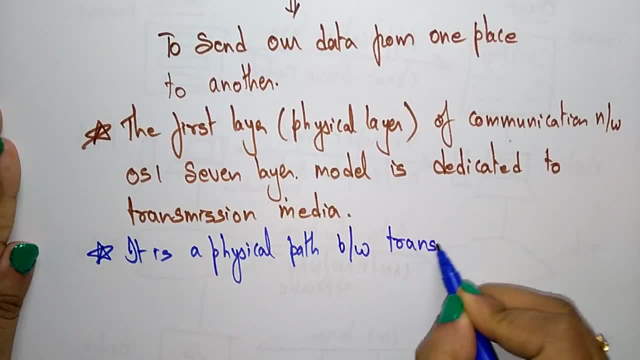 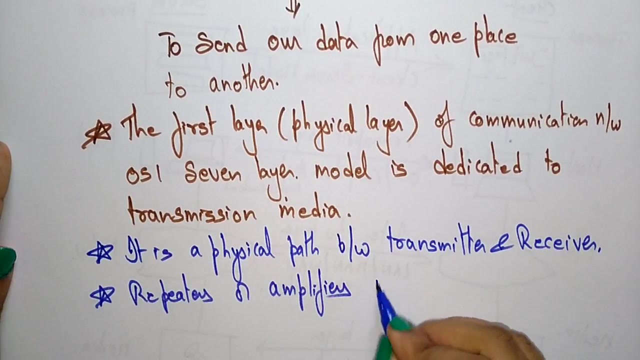 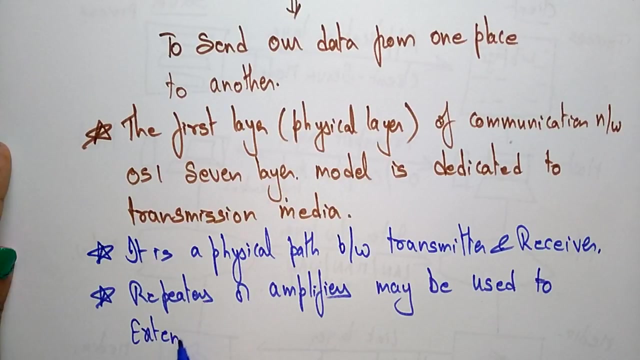 It is a physical path between transmitter and receiver, transmitter and receiver. So to transmit the data from one sender to the receiver, we use repeaters or amplifiers. repeaters or amplifiers may be used to extend the length of media. So to extend the length of medium, you can add more repeaters or amplifiers to send the data from distance. 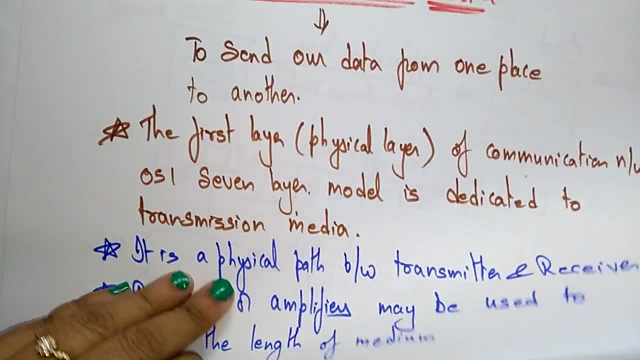 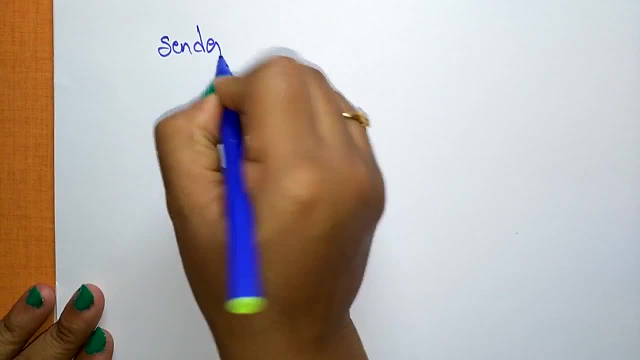 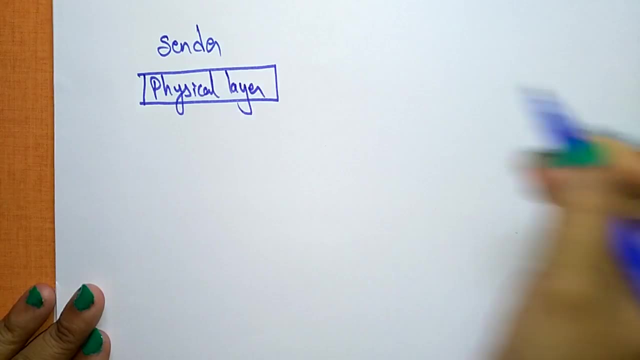 To distance from sender to the receiver. So let me just show you how this transmission media is look like. So let us take this is a sender Physical layer. I am just taking the physical layer from sender side and from the receiver side. So this is the receiver. 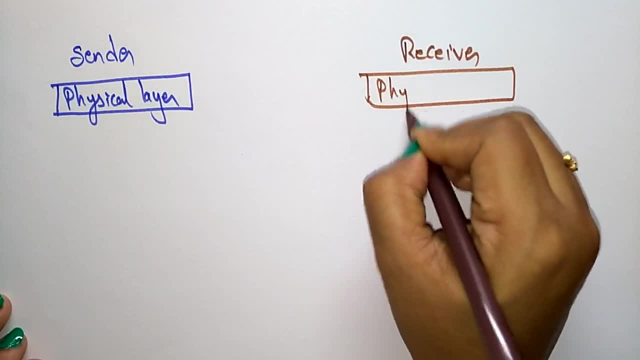 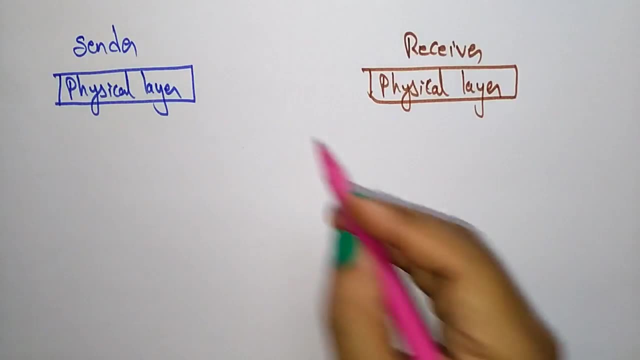 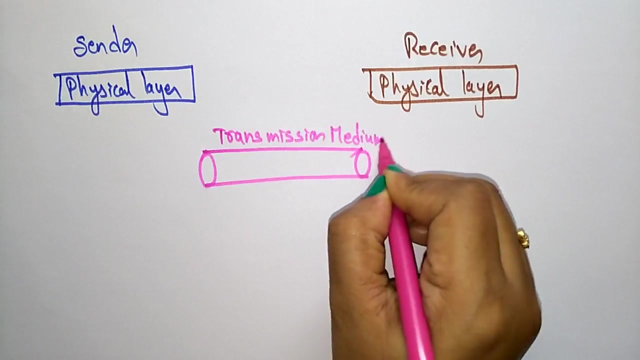 From receiver side also, I am taking the physical layer, Physical Layer, Ok, So in between that we are having the transmission medium. So this is I am taking this is a transmission medium. A transmission medium may be you call it as a cable. 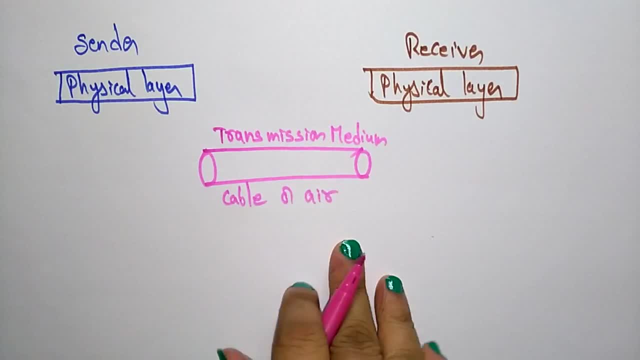 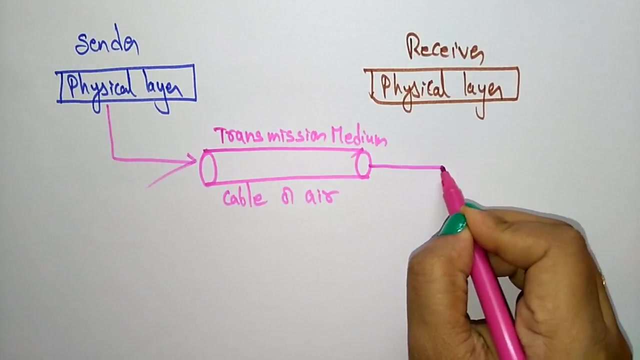 Whether it is a cable or it is in air, That is a wireless. It may be a wired or wireless. You have to be noted that the transmission media may be a wired or wireless. So from physical layer to the cable or air, from sender to receiver. 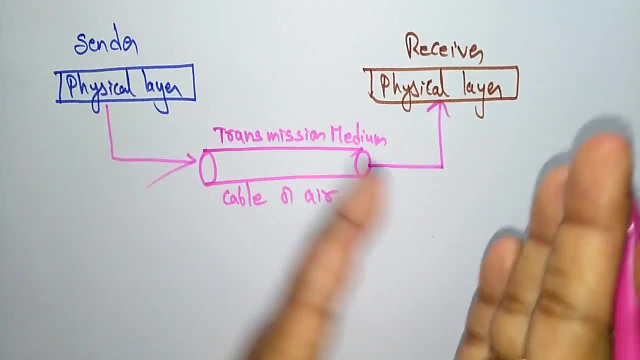 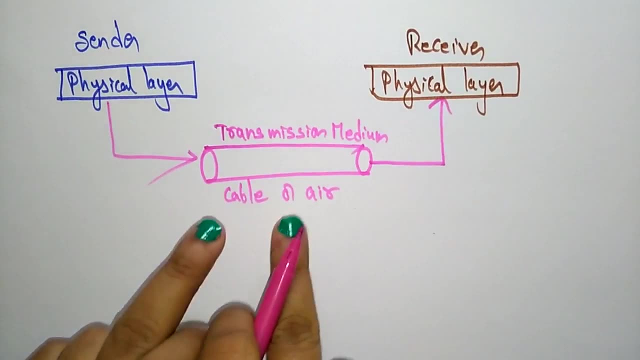 So this is how this transmission media is working: from taking the data from sender and giving the data to the receiver, So with the help of transmission media. So you have to be noted that the transmission media may be a cable or a wireless, That is, it is present in the air. 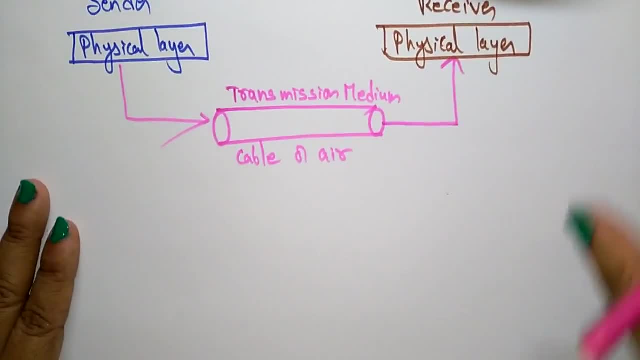 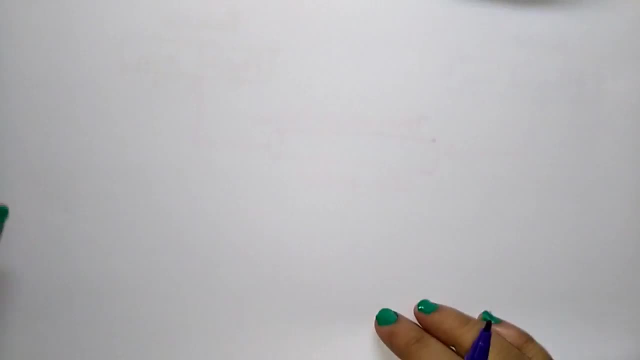 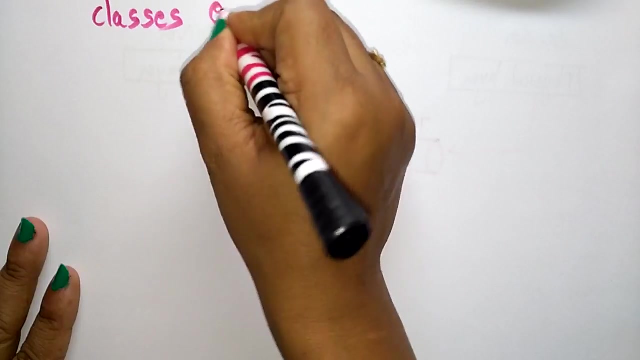 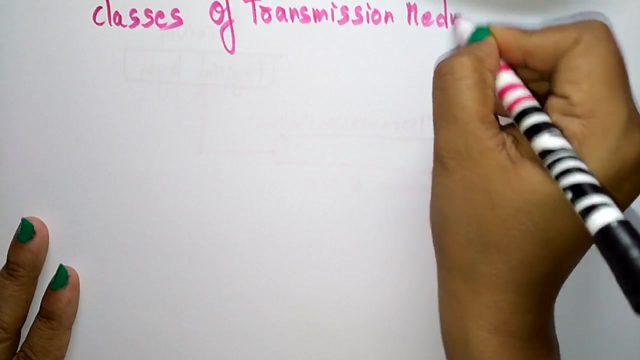 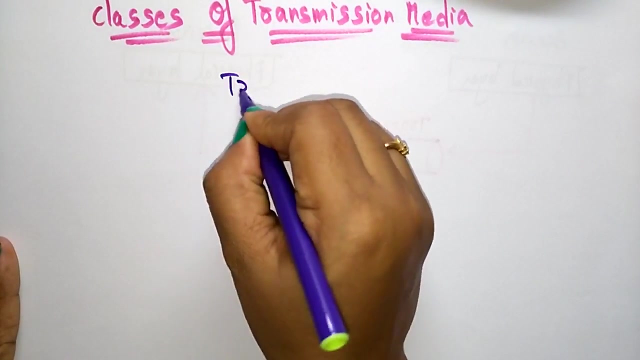 Ok, Now let us see the classes of transmission media. Let me just give a wave: Classes of- I will take a new page- Classes of Transmission Media. So how many types of mediums are there? Let us see. So this is a transmission. 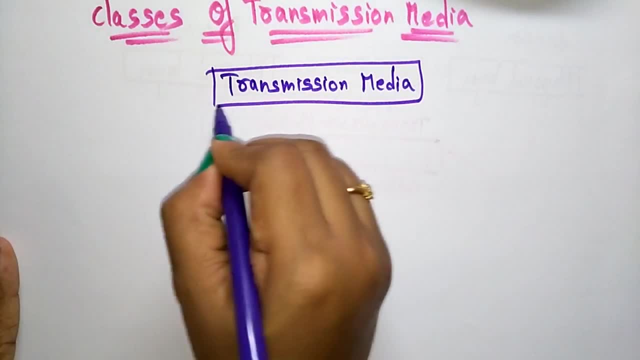 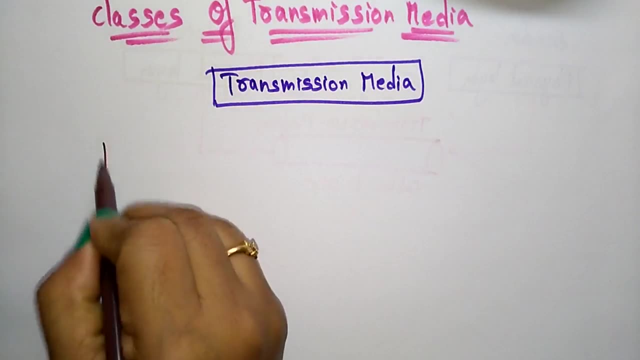 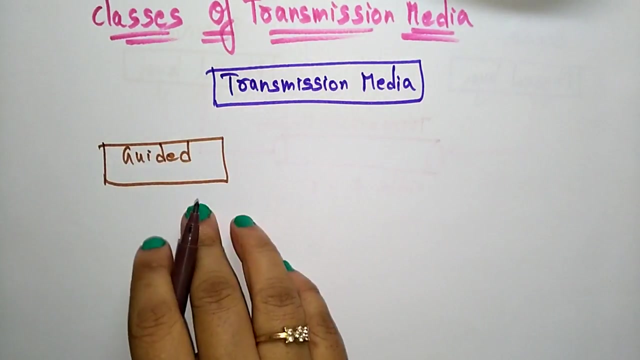 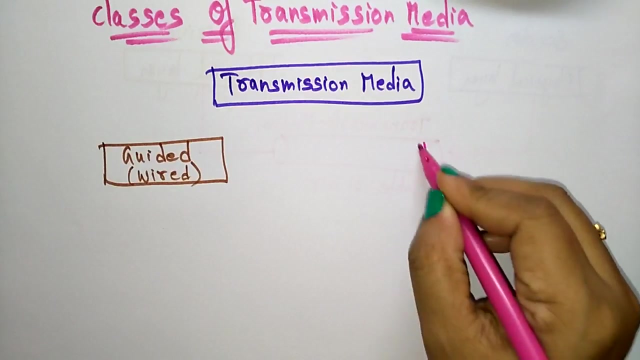 Media. So the transmission media is of two types. Ok, What are those two types? Guided, The transmission media is of two types. One is guided, That guided, you call it as a wired, And another is Unguided. 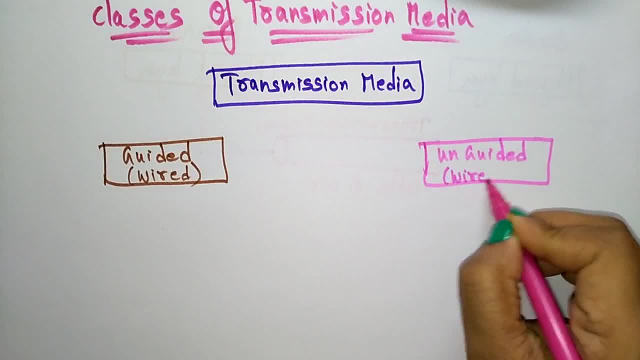 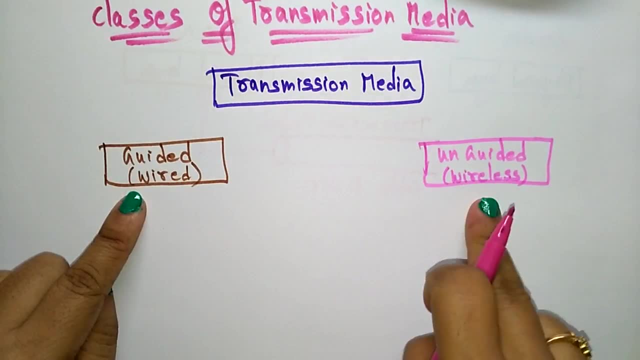 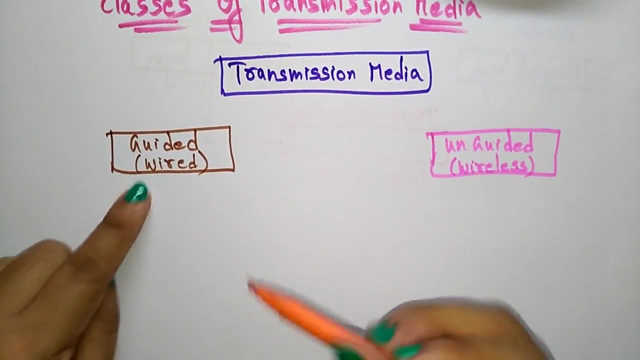 Unguided means wireless. So you have to note that guided media means wired. It is a connection, A physical connection. So unguided means wireless. So a transmission media may be a guide and unguided. So again, this guided transmission media, that is, a wired transmission, is of three types. 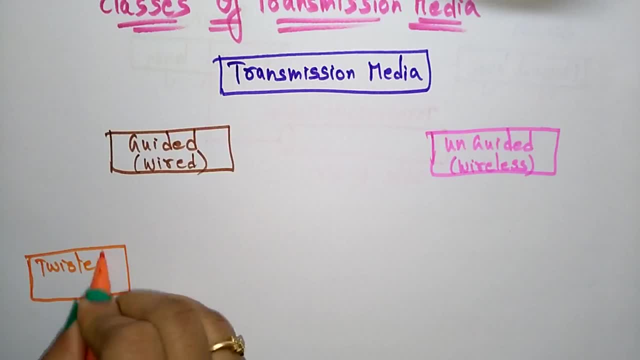 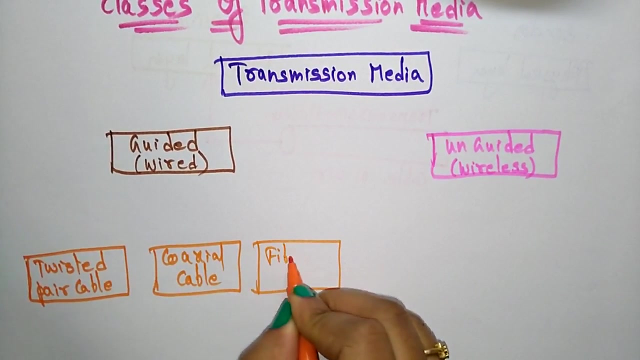 Three types of wires are there, That is, the Twisted pair cable And coaxial Coaxial cable And fiber optics, Fiber optic cable. So these three are the wired cables, Wired media And coming to the unguided 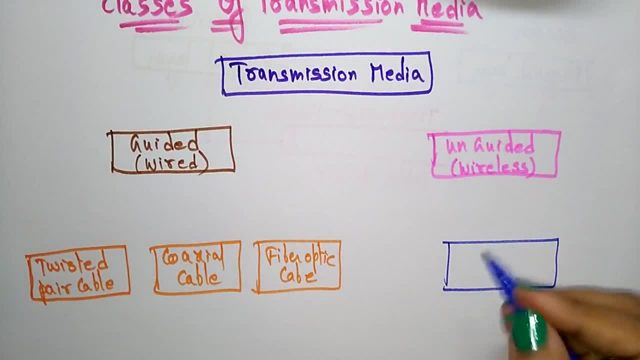 Unguided is just a free space. Wireless- I am talking about wireless, So that is why it is a free space, So there is no physical connection. Free space- So this is a transmission media- is of two types: Guided- 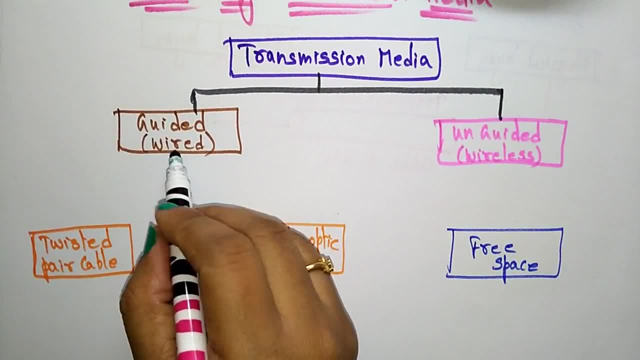 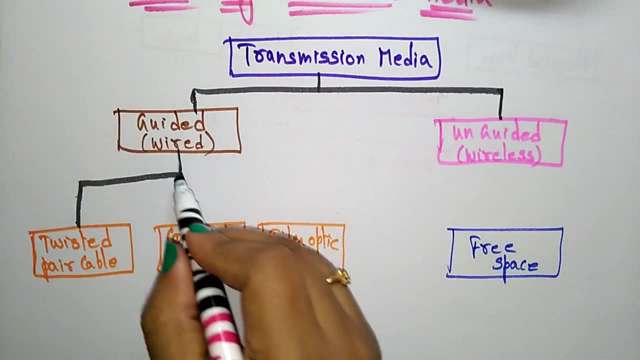 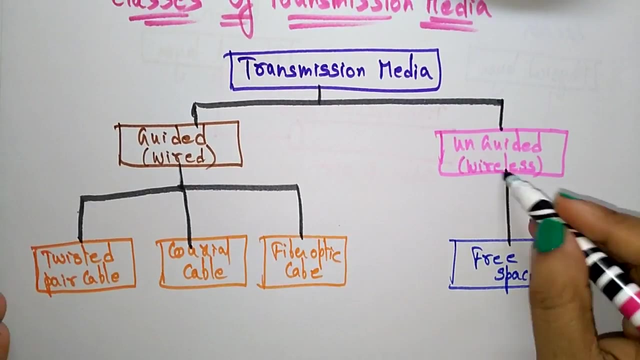 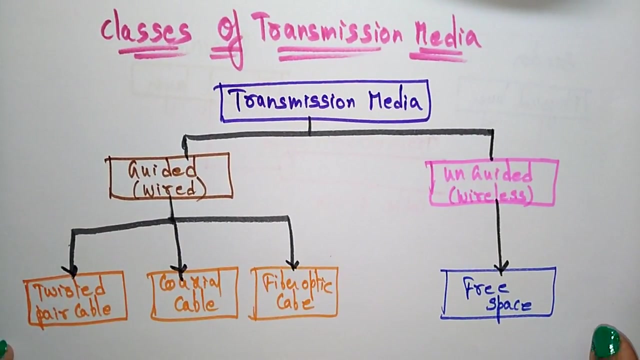 And unguided. So the guided, The wired transmission media. There are three types of wired transmission media: Twisted pair, Coaxial cable And fiber optics, Whereas unguided is free space. Ok, So this is the classes of transmission media. 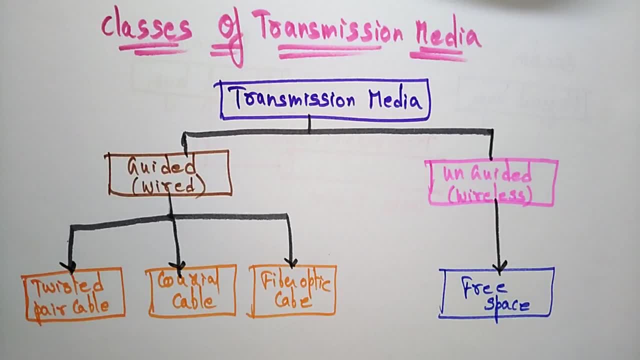 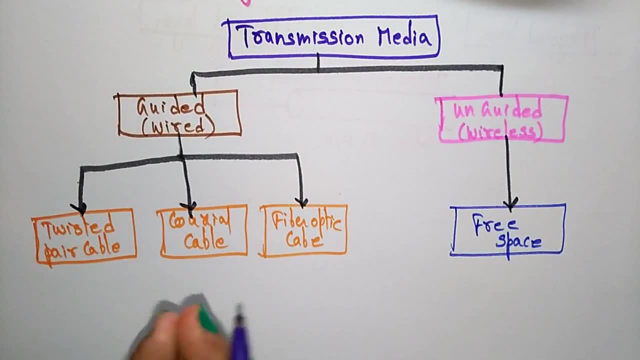 So why we? If you want to select any transmission media, You have to follow some rules. Means, Suppose, if you want, If you want to buy some transmission media, You want to buy some wired cables, Or if you want to go for the wireless. 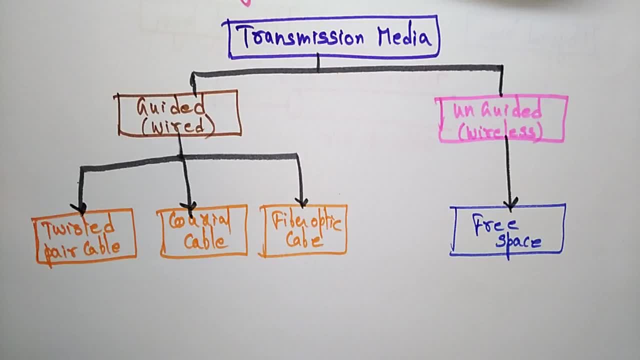 So you have to check some factors, The factors to be considered While selecting a transmission media. So the factors To be considered, or, While selecting a transmission media, The factors that you have to be considered, or So you have to check the. 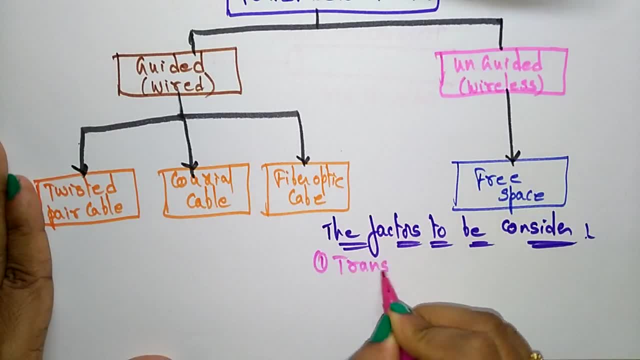 First, transmission rate. What is the transmission rate of that cable That you have to be checked, The transmission rate. And next The cost: The cost of that cable And whether it is easy to install or not, That also you have to be.